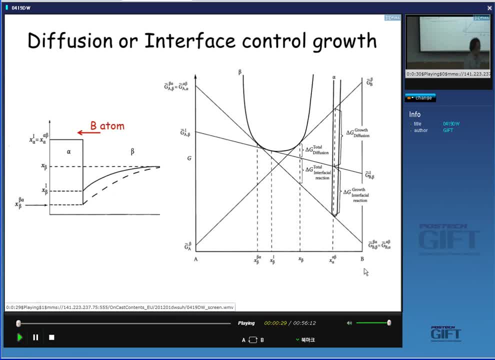 and product pace. The meaning of the local equilibrium is that the concentration at the pace boundary is given by the equilibrium concentration that we can obtain in the equilibrium pace diagram. So I also mentioned that and I also mentioned about the deviation from the local equilibrium When the deviation of the local equilibrium occurs. 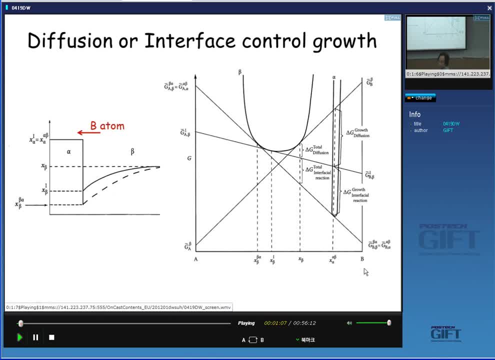 the basic assumption of the local equilibrium is that there is no difficulty for atom to across the interface because there is no difference in the chemical potential across the interface. But sometimes we have to supply the driving force for atom to across the interface. At that case the equilibrium concentration of parents or, in this case, the product pace, is very sharp. 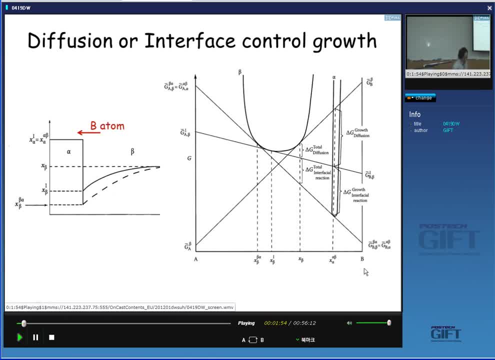 free energy curve, so the concentration is fixed. But in this case we have — the interface concentration have to move along this line To supply additional driving force for atom to across the interface. So, when you assume the local equilibrium, the concentration of 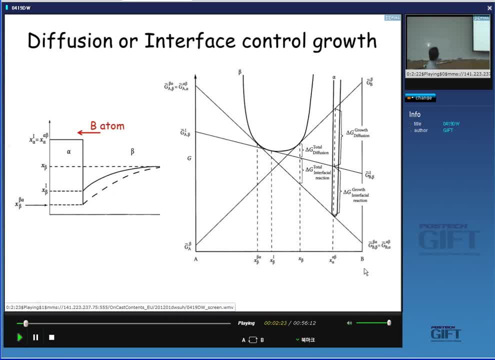 interface given by this point and this point. But when there is a necessity for gevenome, the additional driving force for atom two moves across the interface. the concentration of interface is starting to deviate from the equilibrium value. So in extreme case all of the driving force is consumed by interface reaction. then the 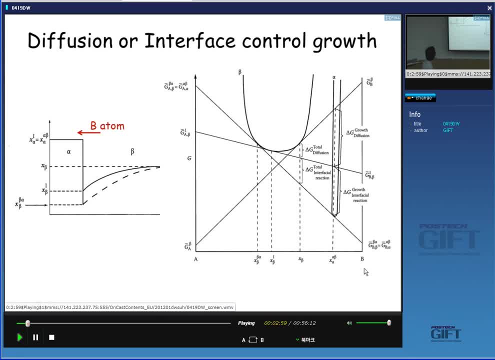 continuous concentration approaches to its original composition. So in this case we call the reaction is purely controlled by interface reaction. But in this case we say it the reaction is diffusion controlled. So from now on I would like to focus on 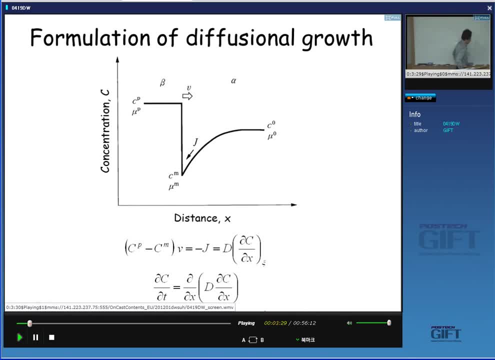 The growth rate of diffusion. controlled reaction means that we assume the local equilibrium between parent space and the product space. Let's think again: the concentration profile during the growth Here, The Beta phase, which is growing inside of the upper, and this is upper phase- and for the 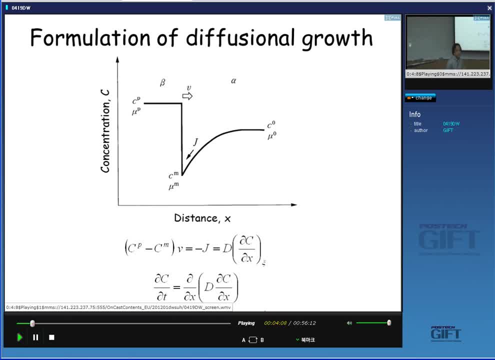 growth, for the growth of beta phase, some amount of atom should be supplied to satisfy the concentration of the beta phase. So the atom should be supplied. This applies to this direction, right, And the supplying of the atom is controlled by the diffusion of that atom in alpha phase. 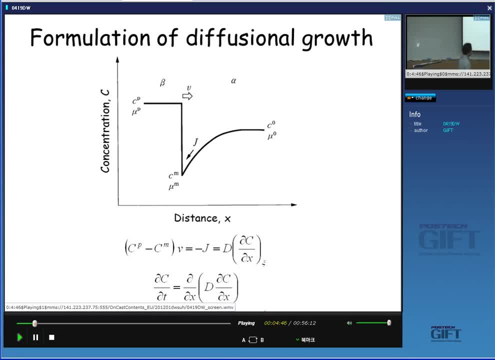 Right. So When We Assume That The Beta Phase Right, So The Velocity Of The Interface In By V, Then This Amount Of Atom Should Be: 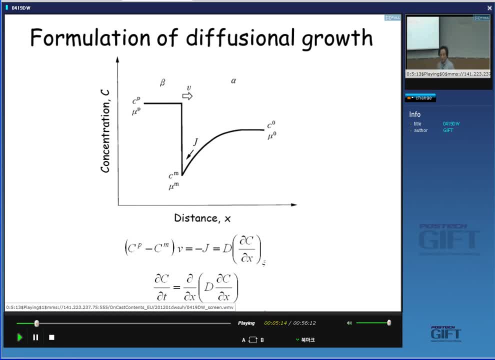 Supplied Per Unit Time, Per Unit Area Of For The Growth Of Beta phase Right. That Is The Difference Among This Point And This Point, And 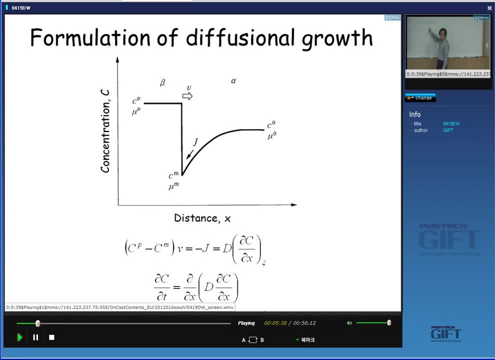 The Velocity Of Interface Is B, So This Amount Of Atom Should Be Supplied. Okay, Everyone Clear. So How Those Kind By Diffusion. So The 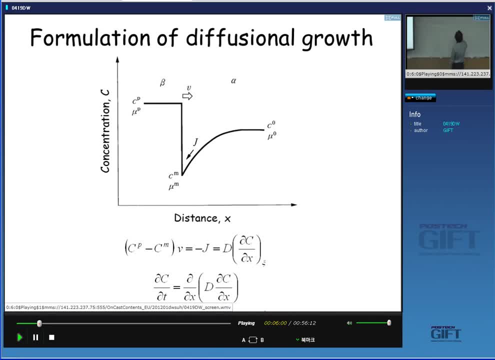 Flux Of Diffusion Is The Diffusion Should Keep Pace With The Growth. Okay, So This Is. This Relationship Is Called Flux Balance Equation For The 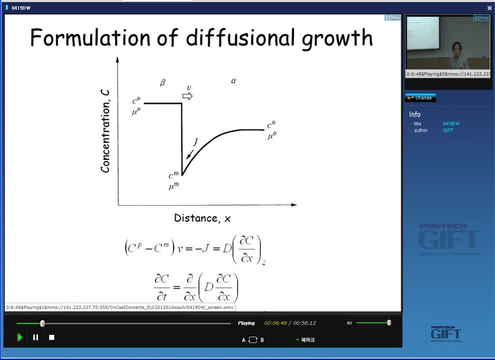 Growth Of The New Pace. The Supply Is Controlled By The Diffusion, So What We Are Interesting Is To Evaluate V When We Know The 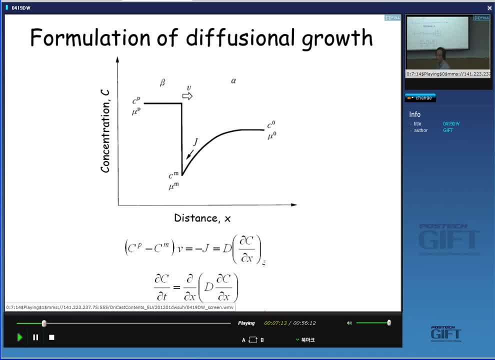 V, That Means We Know The Growth Rate Right. So What If We Know The Concentration Profile Of The Salute In Alpha? Then By Differentiating, 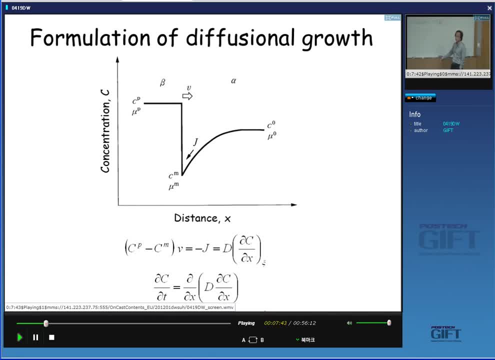 With Concentration, With Position, Then We Can Evaluate The Growth Rate V. That Is The Basic Concept To Obtain The Growth Rate Of The Product. 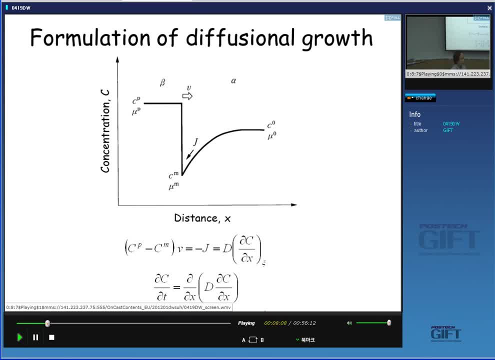 Phase Which Goes By Diffusional Mechanism To Obtain The Concentration Profile. We Have To Solve This Diffusion Equation With Proper Boundary Condition In. 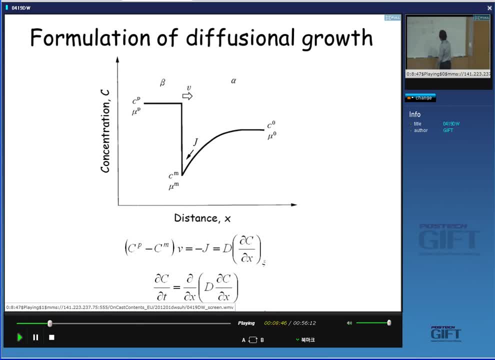 This Case, What Will Be The Boundary Definite? C Goes C, Zero, X Goes C. C Means That The Position Of The Interface When X. 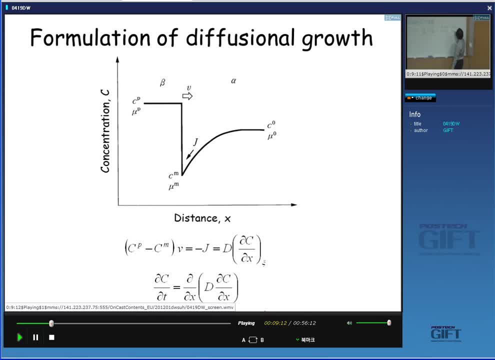 Goes To C, Then Concentration Goes C, M Right, So With Concentration, And Then Put Concentration Profile To Flux Balance Equation, Then Finally We 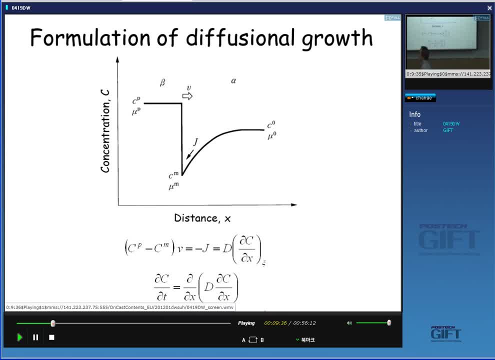 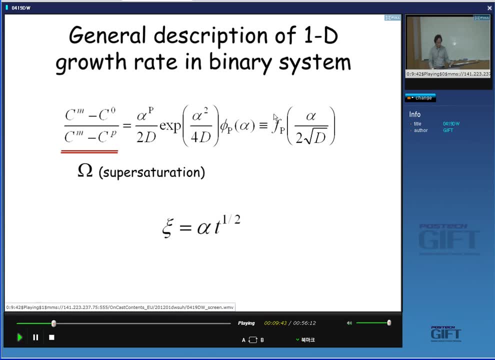 Can Get The Growth Rate Okay For The One Dimensional Growth In Binary Alloy, So We Alloy. The Growth Rate Is Given By This Formulation: 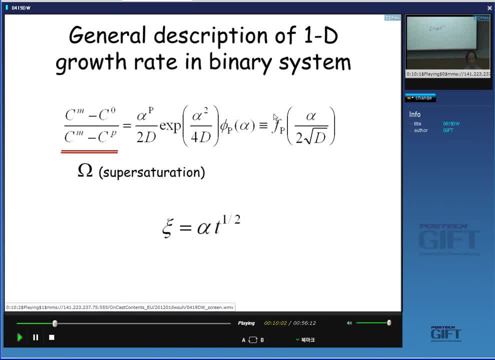 So In This Class, What I Want To Do Is Drive This Formulation When You Look At Just The- If You Know The Page Diagram. 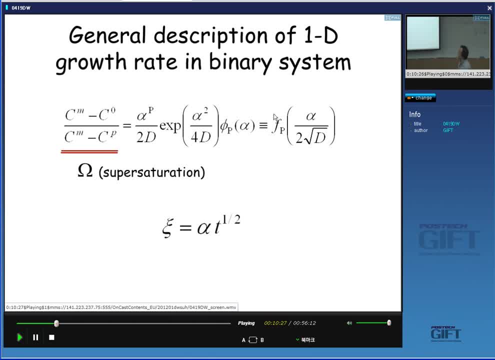 You Can Easily Evaluate This One. This Is Given By The Concentration Of The Page Boundary. So This, When Temperature And Pressure Is Here, P. 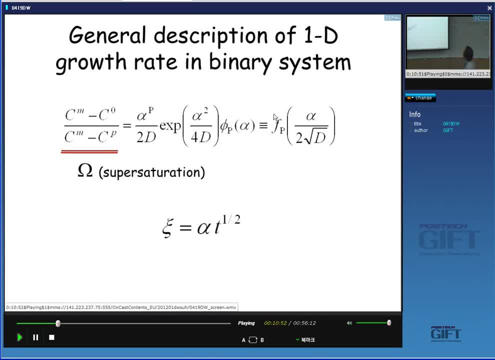 Is A Constant. P Is A Constant Which Is Related To The Geometry. When P Is One, This Equation Is Plana, Plana Gross. When P 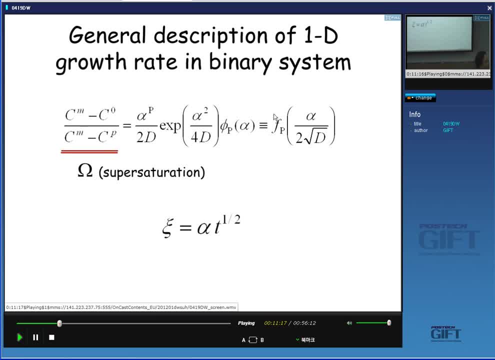 Is Two. It Is The Gross Of Spherical Shape Product Phase, So You Do Not Have Any Concern About P. So Actually This Is A. 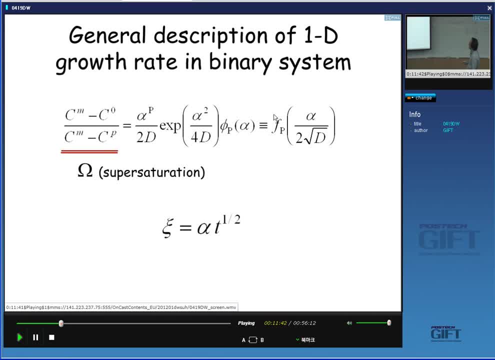 Non Linear Equation About Alpha. So The Meaning Of The What? The Meaning Of Knowing Alpha Is That We Know The Position Of The Interface With. 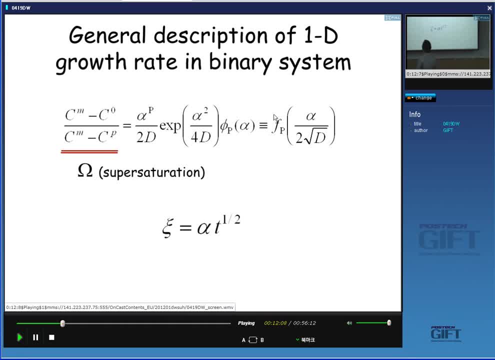 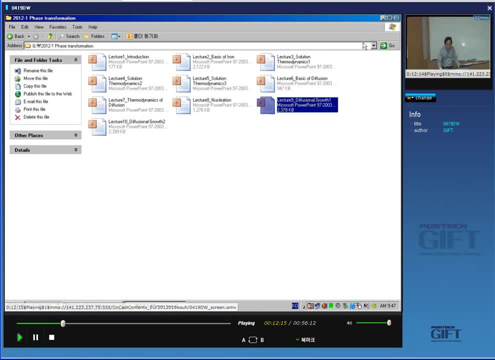 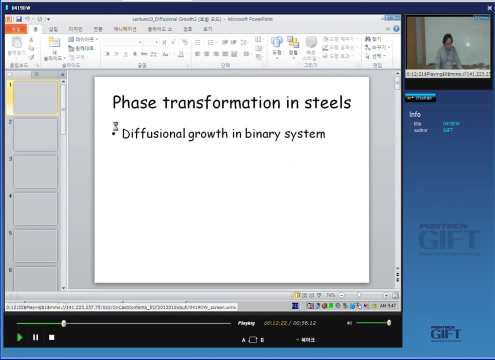 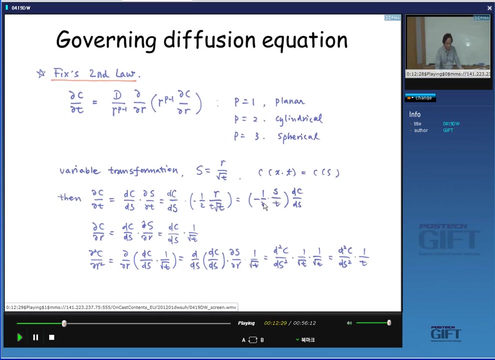 Respect To Time, So We Can Evaluate The Gross Rate Of The Equation. About Phase: So We Can Have Any Concern About Phase, About The Equation. 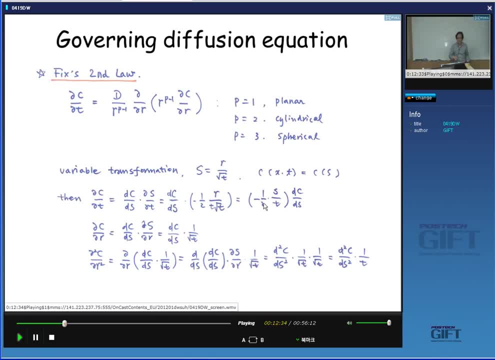 About The Interface, About The Interface, About The Interface, About The Equation, About The Equation About The Interface. We have Some Others, Yes, So We have About what? 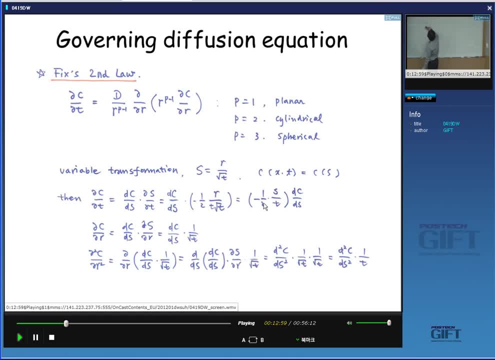 You Think Together In That Package Of A Figure There. So On This Layin The Certainly Add Some We some explanation to help your understanding Here. this is fixed. second law: 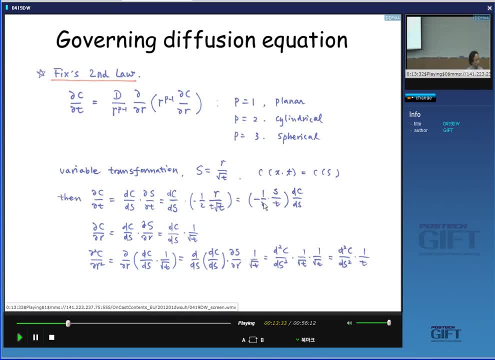 and this is governing equation We have to solve right. So this is so much like different form from the usual value, but it is simply the same when you put one, two, three as a geometric vector. So when you put one, you simply have. 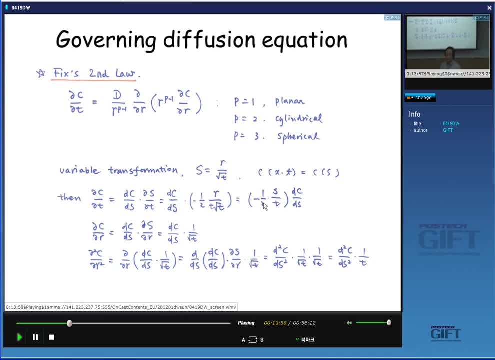 the form you are familiar with. And when you put one, you simply have this kind of one-dimensional fixed second law. And actually, when you put two and P, three, and this equation becomes the governing equation of the diffusion in cylindrical or spherical shape of the product phase. 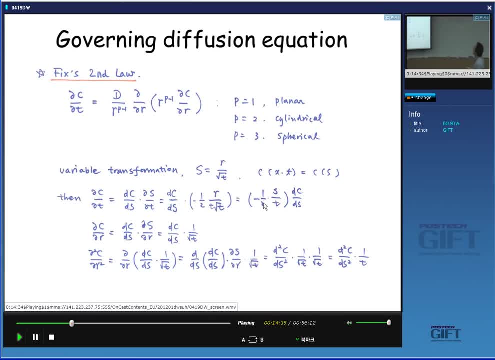 Anyway, this is a general form, so let's start with this, Then we can expand and speak in whatever discipline model we have, depending on the geometry of the product phase, why we have to put, why we have to do those kind of variable transformation. 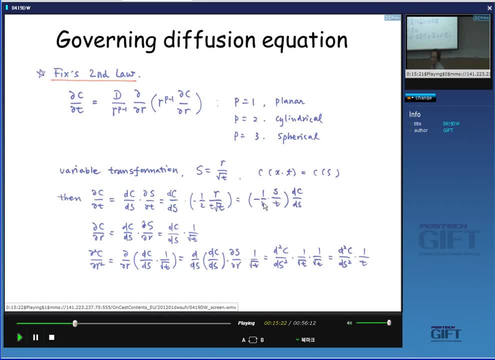 Actually to solving the partial difference. location is a kind of the experienced way. So many times ago many mathematicians- the people who work on mathematics- tried many ways to solve this kind of equation. So they finally found if we make a variable transformation like this one, we can solve. 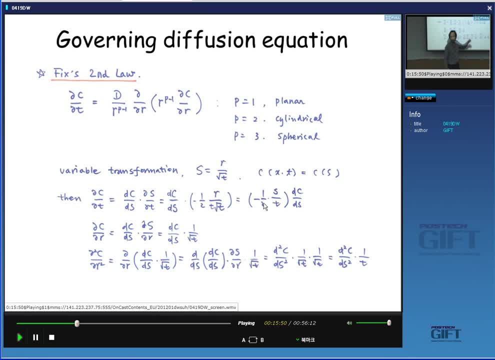 it. Actually, when you look at the final form of the solution, then the variable r and t always should have this kind of relation. Otherwise that cannot be a solution of this diffusion equation. So let's start with this variable transformation, Then the concentration which depends on position and time will be a simple one. 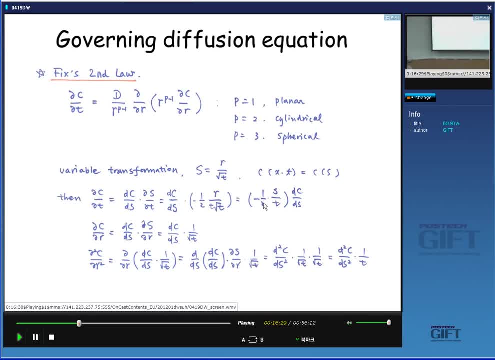 variable function, right. So with this relationship, let's try partial sheet over partial time with this chain rule. Then the concentration first derivative of concentration, first differential of concentration with respect to time, Then you can have This kind of form by chain rule, okay. 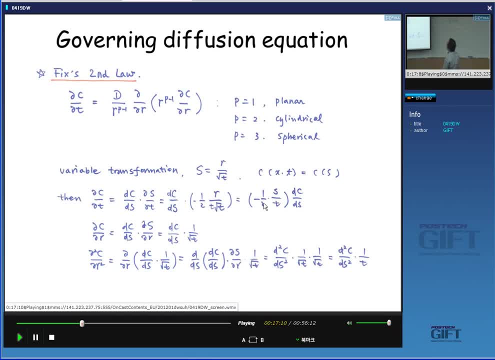 And secondly, the concentration with position. r is the same meaning with the x, but we write r for more general concept. Usually x means What? Just one thing, Just one dimension, right? So anyway, if we evaluate this term, you can have this one right. 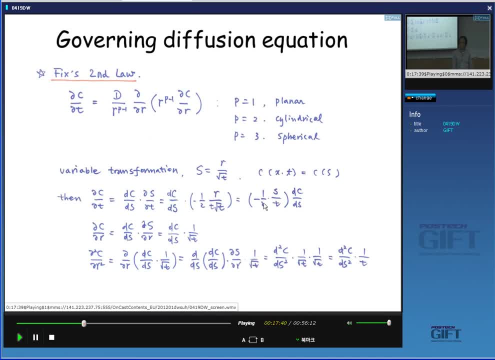 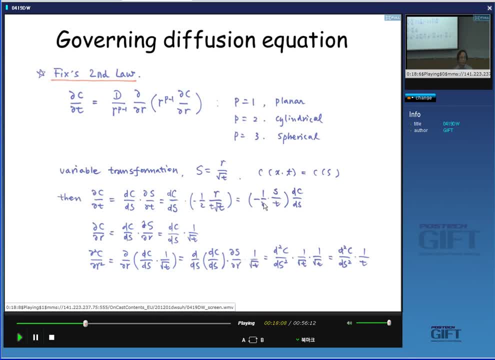 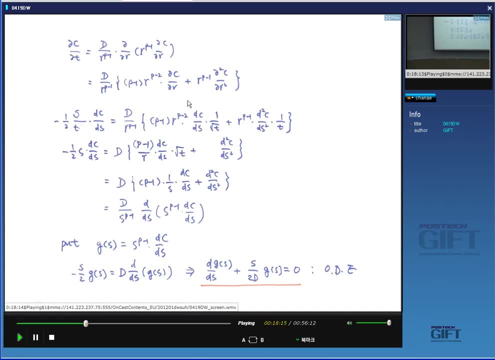 But for our basic equation. the fundamental equation is: when we add all the variables to this equation, then it's rid of x. It's very simple. So for a simple equation, use this variable and add only one variable section to it and you can have this equation and, after some arrangement, finally you can have this kind of. 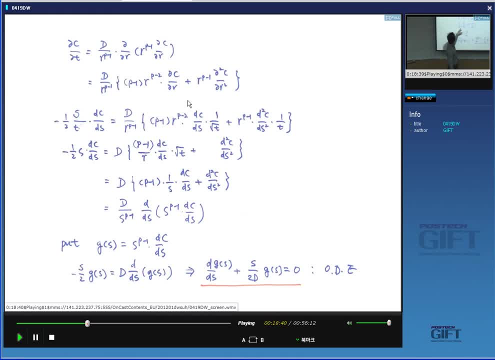 form with this one. It looks complicated, but if you follow the formulation once then you can easily understand. With this relationship, if you put this term with another function- GS, just put the name of the function- then this relationship converted into this form. 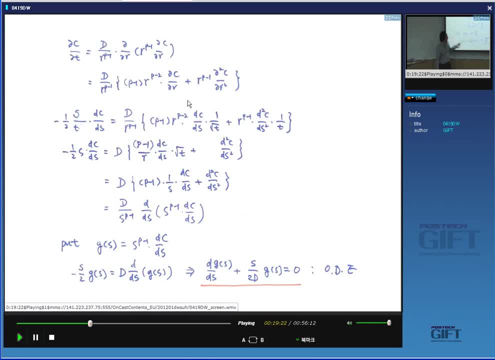 And for, And. finally you can obtain this equation. So now we convert the partial difference equation into ordinary difference equation. The procedure seems to be complicated, but it's a kind of mathematical skill, So I think you do not worry about it. All of you are smarter than me. then you have no difficulty to follow. 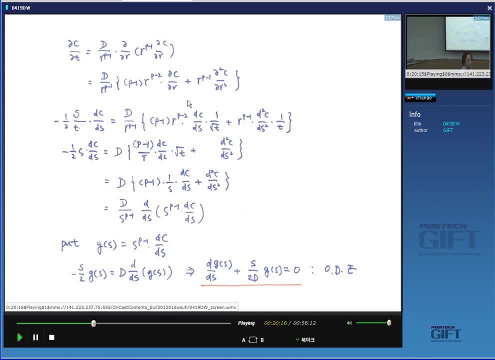 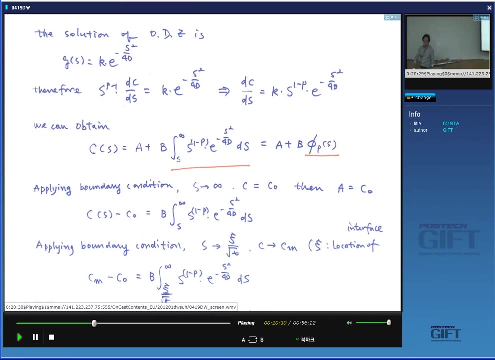 Any question? No, Okay, So what we have to do is to solve this ordinary equation, ordinary difference equation, And the solution is already given. The solution is given by this exponential term. So the ordinary differential equation is ds, dgs plus 2d over s gs equals 0.. 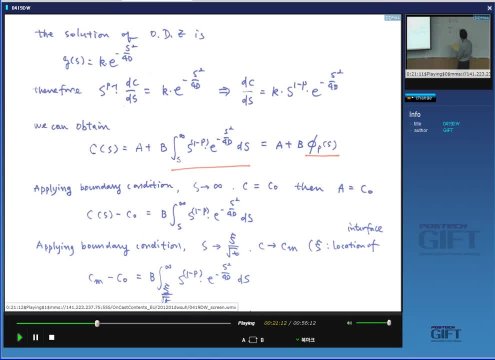 And gs. when you solve it, gs is 0.. So the ordinary differential equation is: ds, dgs plus 2d over s gs equals 0.. Just m out and exponential 4d over s squared, You can confirm whether this is the solution or not. 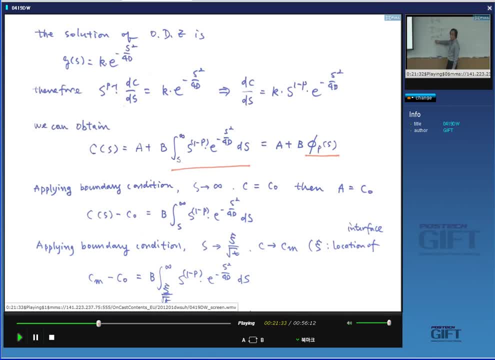 Or just put this value into this original equation. Just put this value into this original equation, Then you can find this is the solution, Then you can find this is the solution. All right, Here Eva gives the difference. Okay, It does. 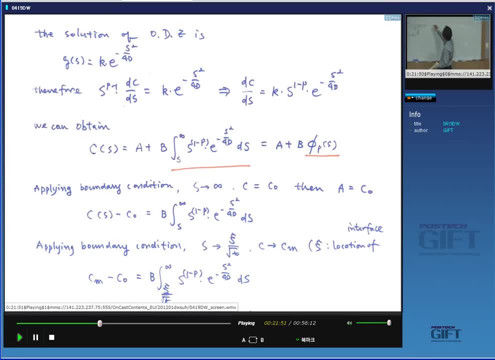 All right, Herelow to zero, Right Here, bottled, Okay, Okay, All right. gs is originally has the form p minus 1, bs over dc, all right. So when you put this to this, then c and c is ks1 minus p, exponential minus 4d over s squared. 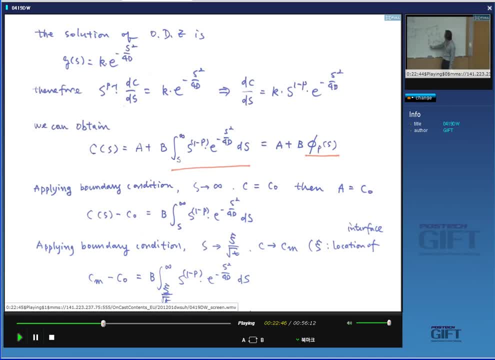 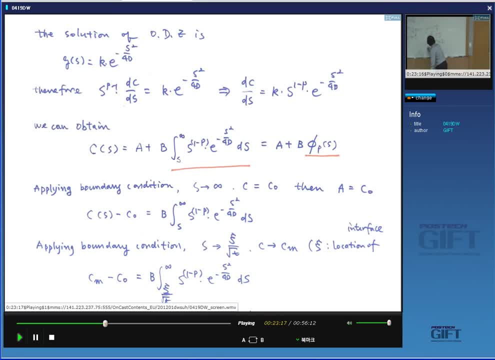 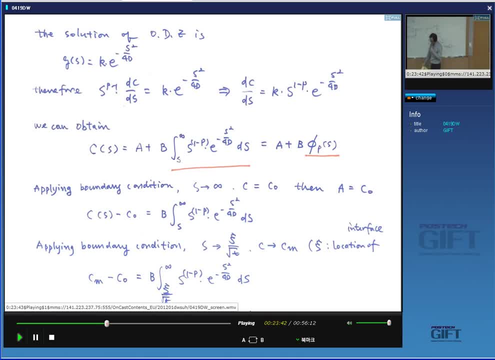 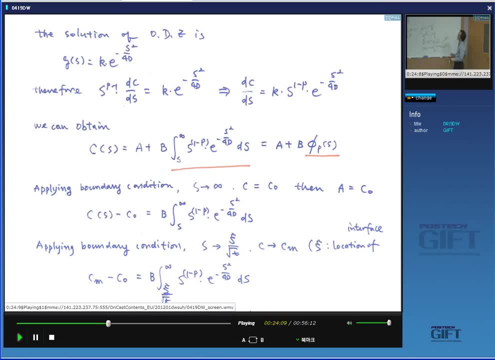 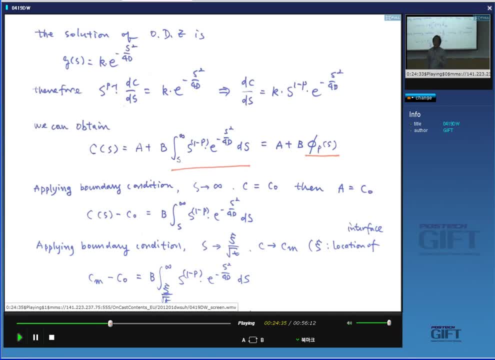 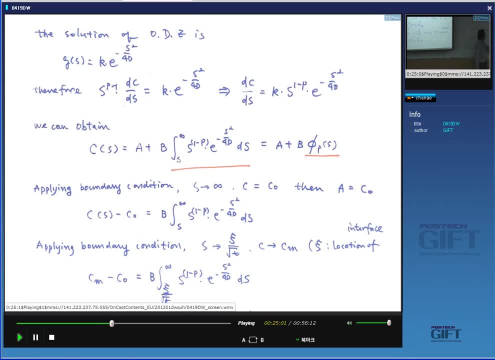 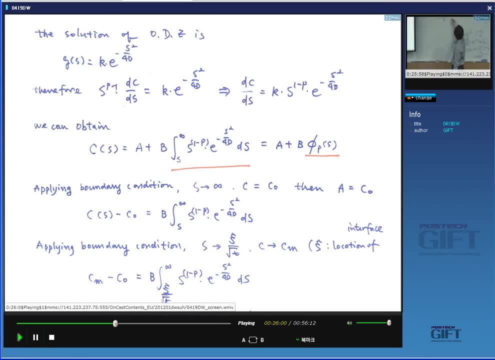 Then c goes, cm, right, Okay. So here, when s goes approaches to infinite, this term will be zero, right? So the constant a should be c Zero, Okay, Are you clear? Are you clear? So c? s goes c zero, b s, so minus p exponential. 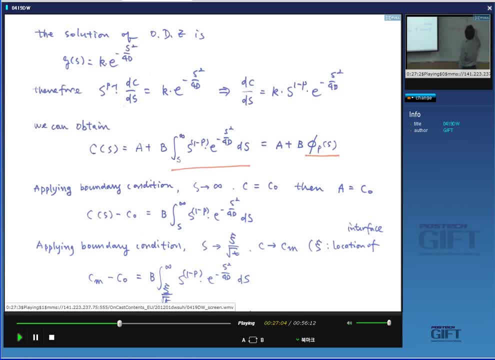 and then c? s goes, c zero, b s. so minus p, exponential S squared bs, S squared bs. Here you have noticed that this value- Cm minus C0, is constant. when the temperature is fixed, then that value is given. 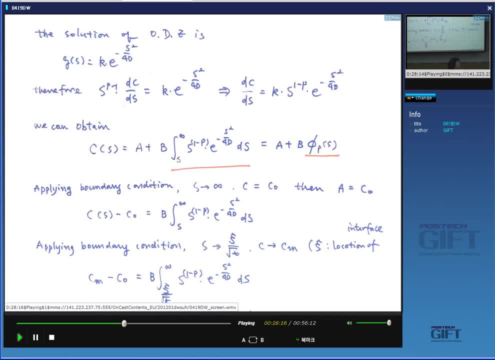 by the concentration of the boundary phase boundary right. This, when we rewrite this one, this is given by this right, So when the temperature is fixed, you can obtain these two values from the phase boundary, which means the equilibrium concentration. 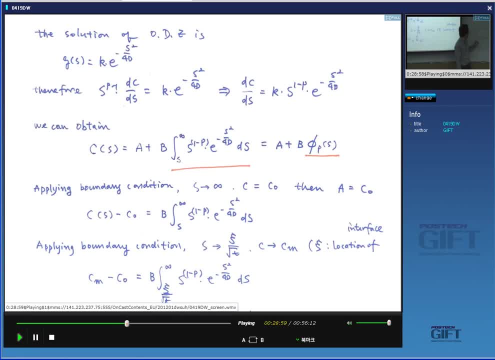 So this Cm minus C0 becomes constant. So that means that this value, the integration interval, the starting of integration interval, should be constant. Okay, Okay, Okay. Are you clear, Not clear? Clear? If this value is not constant, there is no way for this term become constant, right? 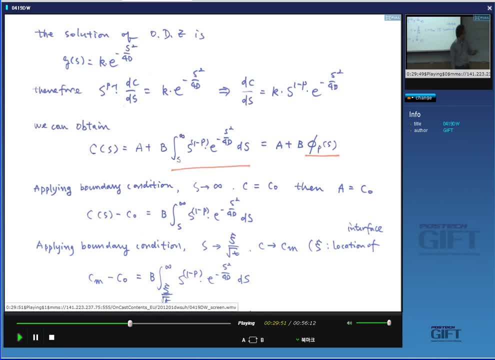 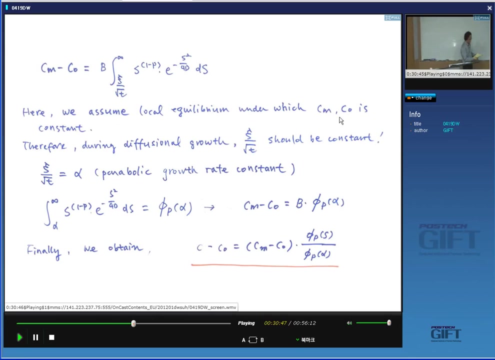 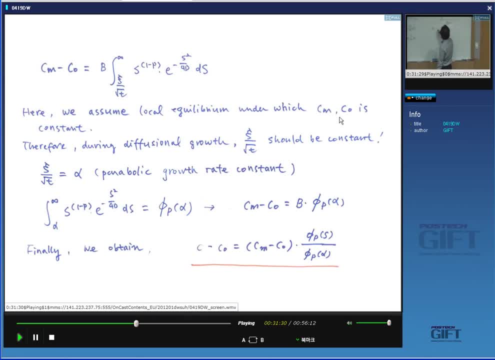 will c m minus c g o pi p r. Okay, Ah, reversed. So the final form of the concentration will be c equal c g o plus pi p r power. c m minus c g o pi p s. This is final form of of our concentration profile. 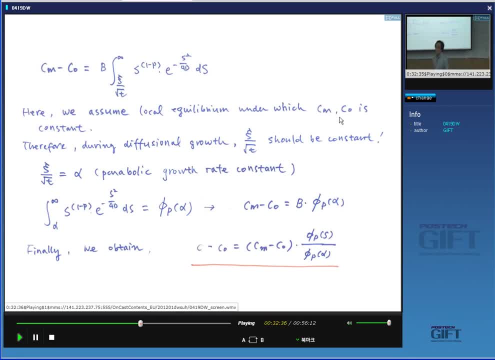 So now we have concentration profile. So what is the next stage? Sorry Yeah, we have to apply this concentration profile to the flux balance equation to obtain the velocity. So here's the velocity. So we're trying to find. 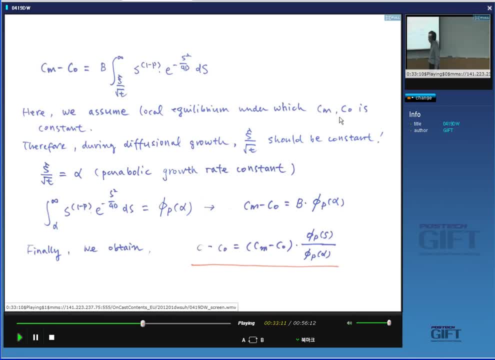 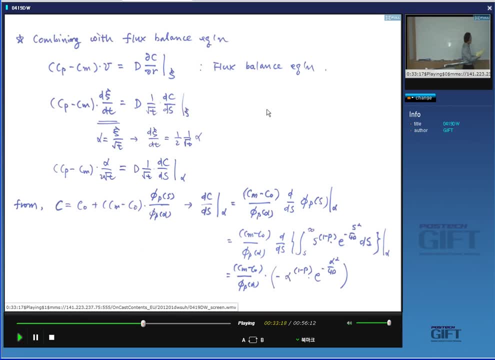 the velocity And we're trying to find the velocity of the flux balance equation. So here's the velocity of the flux balance equation. So we can say this is c, p, over, c, m, v, r, c, p, v, go, d, partial, c, c. 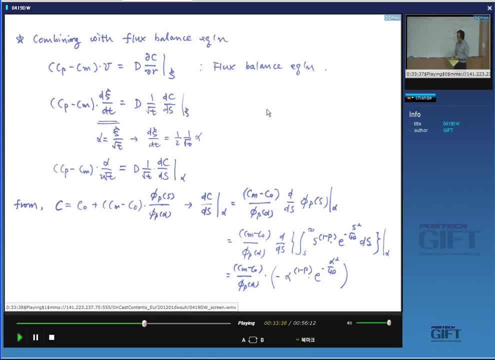 Here again the psi means the position of the interface, So here the v is derivative of position with respect to time. right, If we put the position of interface psi, then when we take the first difference with respect to time, then we can obtain the velocity. 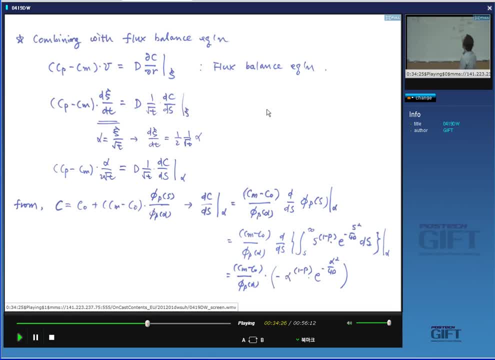 And this is 2 root of t over. that's correct alpha, Because alpha root of t. So when you take first difference with see, with time, then you can obtain this one. So now we are here, Then what we have to do is that. 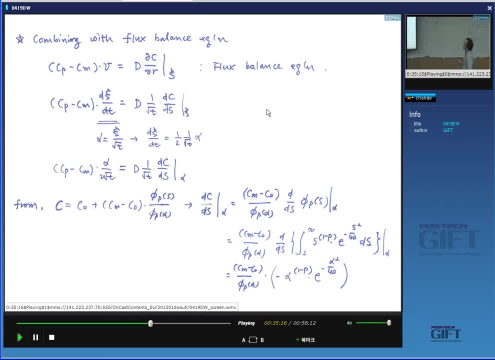 evaluating the first derivative of concentration with respect to value of s at position psi. Now we already know the concentration profile is given by this one. And take the derivative with respect to s. This is constant, so it will be disappear And this is here. 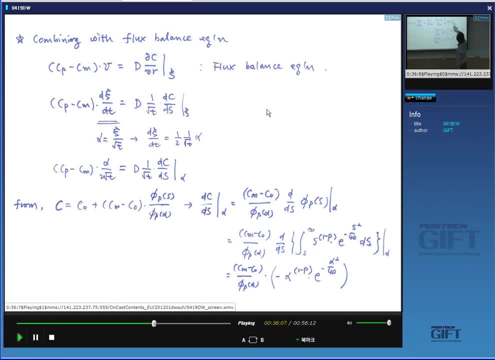 And the only thing you have to do is evaluating the derivative pi p with respect to s at position alpha. Come on. 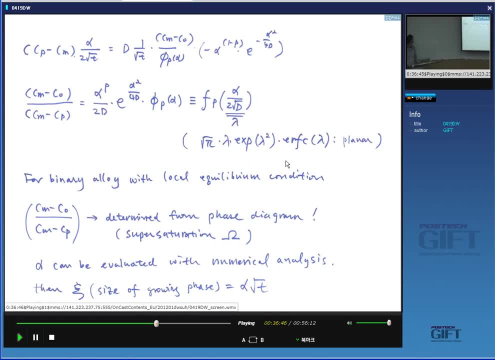 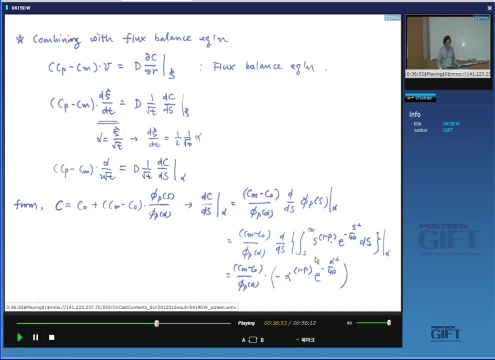 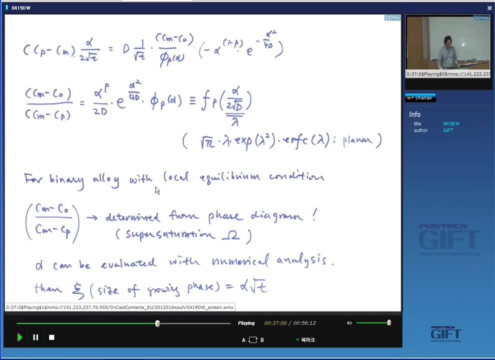 So by arranging with this one, By arranging this one, you have a binary. You will have this formulation. That is exactly the same formula I show you at the beginning of this class. So now you can understand the. 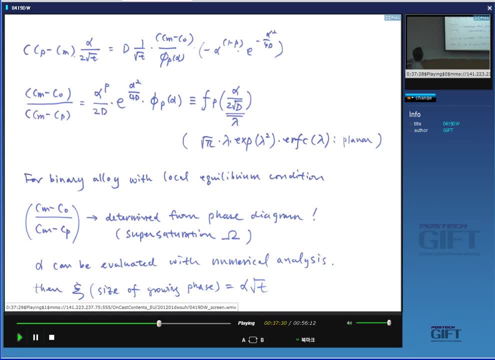 meaning of p, alpha, and pi, p and so on. So, as I mentioned, in the binary alloy system, you already know this value, which is called super saturation. So this: when this is fixed, then the only thing you have to do is to solve this nonlinear equation with respect to alpha. Then, when, 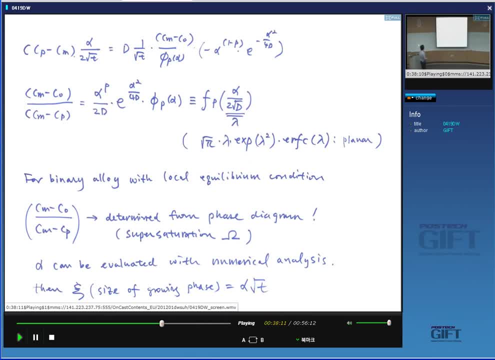 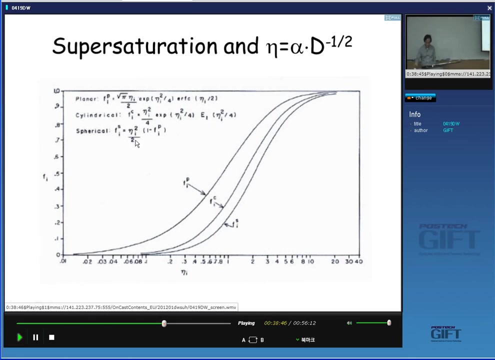 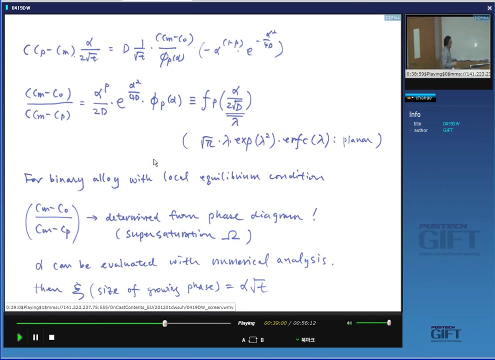 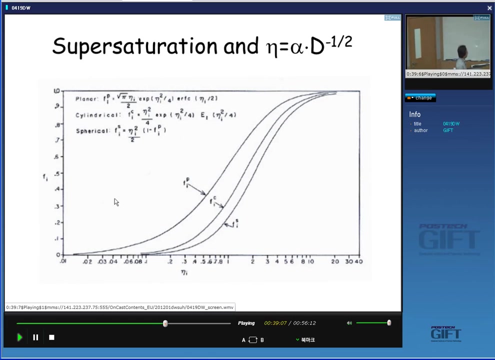 you have alpha, you can evaluate The location of the interface with this and everything is solved. Any question? Yes, Here this graph I copied from some papers And this is actually. this is omega, which is the degree of supersaturation. supersaturation Because the author is different, so they use. 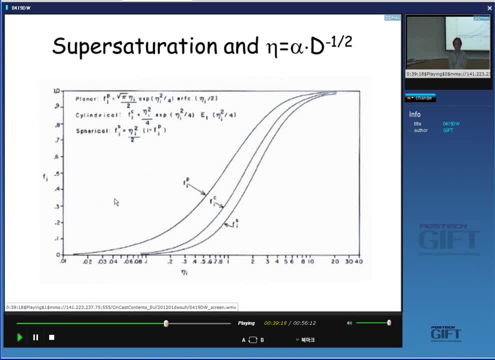 different nomenclature, different character for indicating the supersaturation. And here eta is alpha over scale root of d. It is scaled alpha scaled with the scale root d right. So when we plot the eta which is related to alpha right, Alpha means the growth rate. 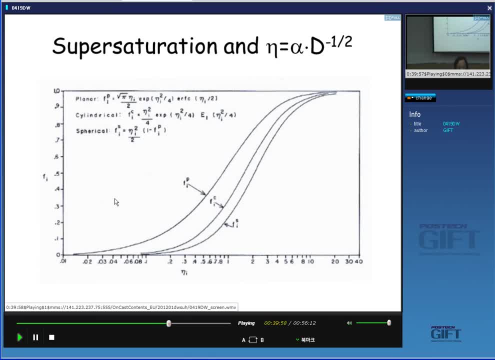 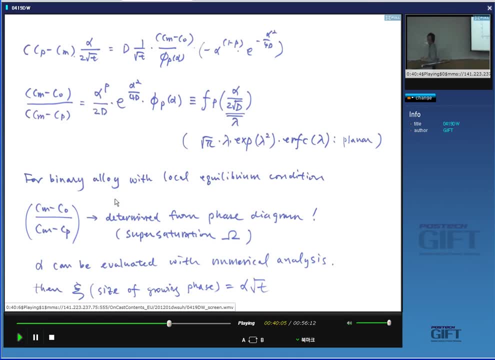 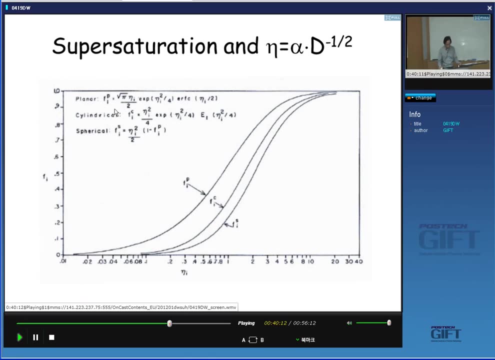 indicating the growth rate, the constant indicating the growth rate right Here, alpha right, We called it as a parabolic growth rate constant. So by plotting, by solving the previous equation, you have this kind of curve which indicating the growth rate constant with respect to the supersaturation, As you can expect, 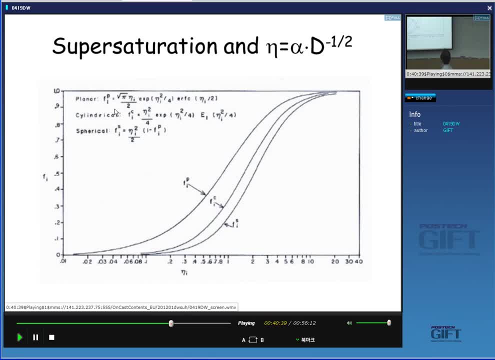 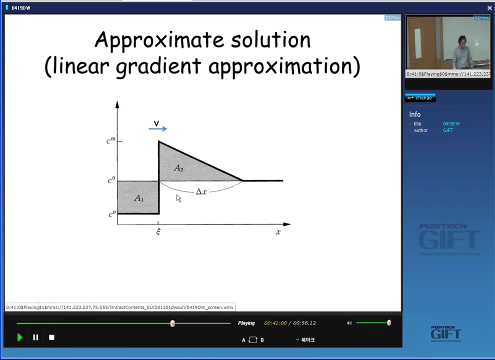 the degree of supersaturation increase, then the growth rate increase. Okay, Because those kind of the derivation of the exact solution is quite not difficult, but I think it is stands out for its kind of time consuming. Sometimes you want to. 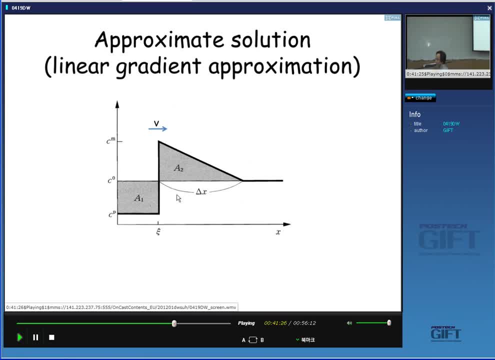 very quick evaluation, but not that exact, with less accuracy. So for that purpose we often use the linear gradient approximation which is proposed by Genner. So you are familiar, very familiar with this kind of 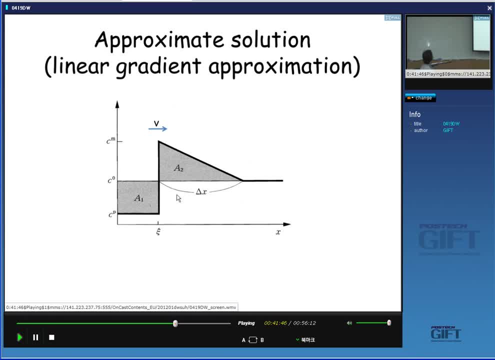 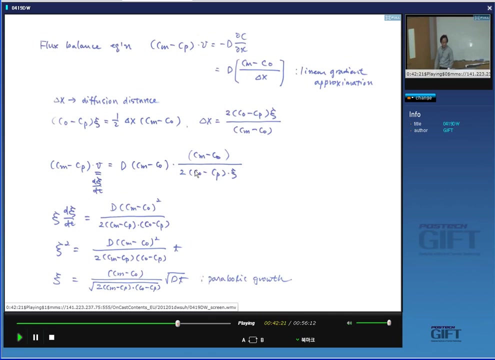 approximative solution. Here we assume that linear concentration gradient ahead of the interface. By assuming this linear concentration gradient, the situation you have to handle is incredibly simplified. So, starting with flux balance equation, you are already familiar with this equation. 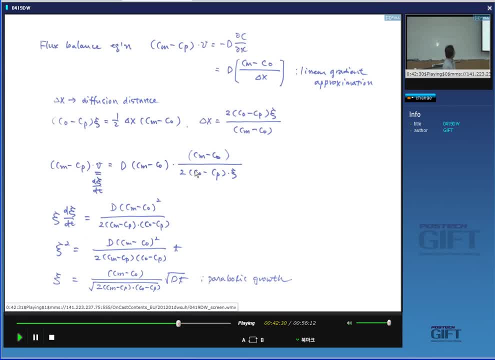 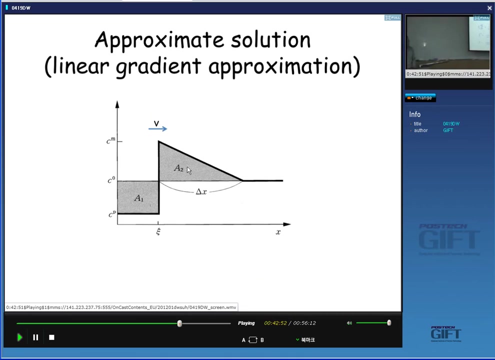 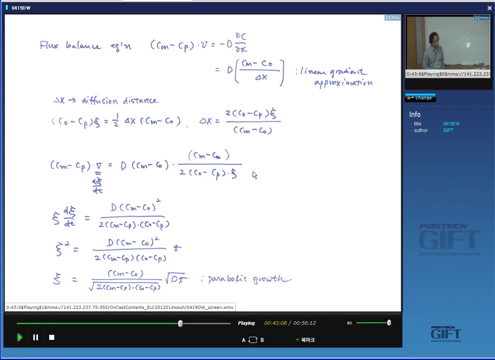 and because we assume linear concentration profile, so it can represent with this one Here x is the length of diffusion area in previous slide, This one. So the only thing you have to do is to evaluate that diffusion length. Then you can evaluate free with this term. 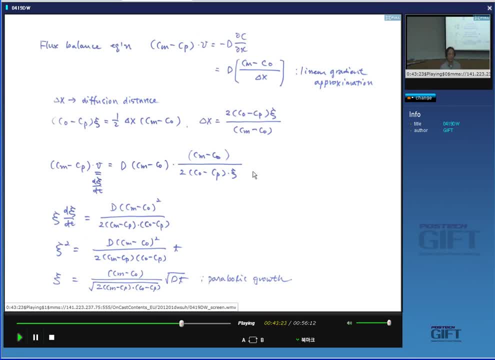 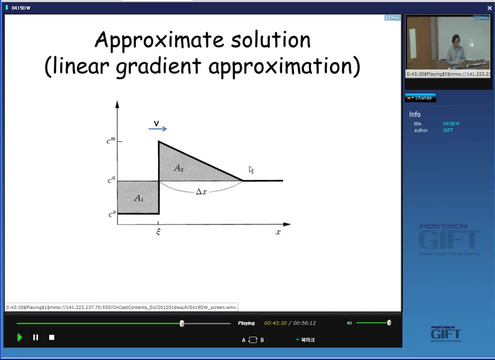 So the way to evaluate diffusion length is that these two area should be the same. The amount of solute which diffuse out into parent space should be the amount of solute accumulated in parent space, right? So by creating these two area, 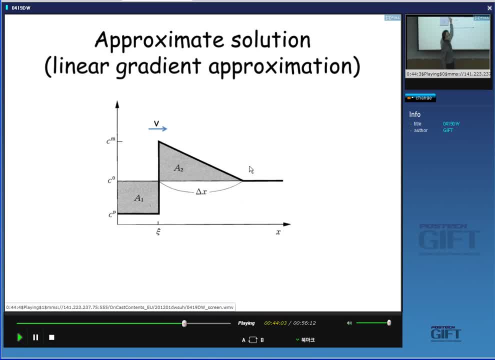 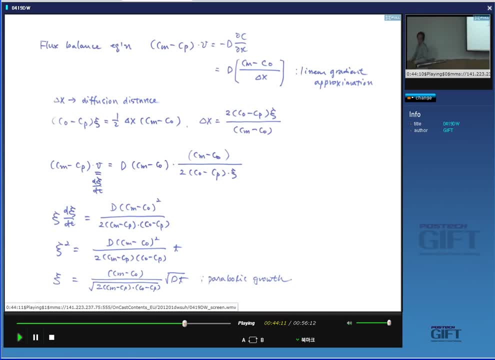 you can evaluating the diffusion length. So here is the relationship and from this relationship you can evaluate delta x, which representing the diffusion length, And just put this value to this equation and rearrange the flux balance equation. Then, finally, you can have this kind of form: 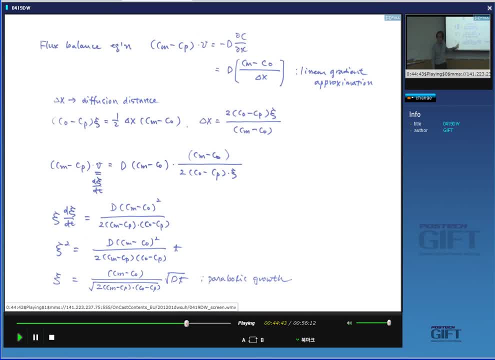 Surprisingly, even though we have very simplified approximation with linear concentration gradient, the final form is very similar to the exact solution we just derived Here. you can understand this term except scale with the t. this term give you the parabolic growth rate, constant alpha. 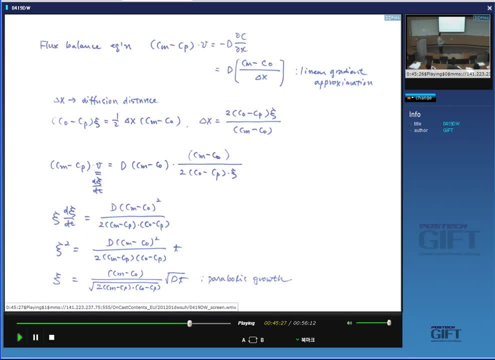 Okay. So even though we assumes very simplified form of concentration gradient, the underlying physics can be taken To make it very clear. the behavior of the entire application can be captured. The movement of interface is proportional to the scale root time, which means parabolic growth rate. 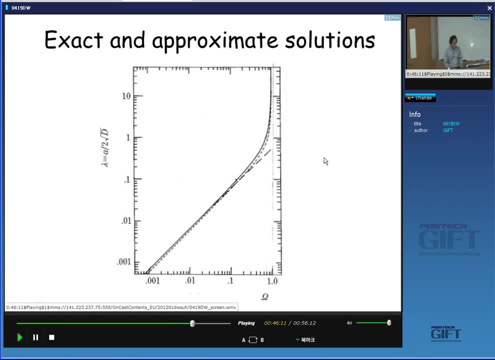 Parabolic growth. Those kinds of concepts can be captured even with a simplified approach. So here we compare the exact solution and simplified linear concentration gradient. Here the solid line represents the exact solution and this dotted line indicating the solution from the approximation. 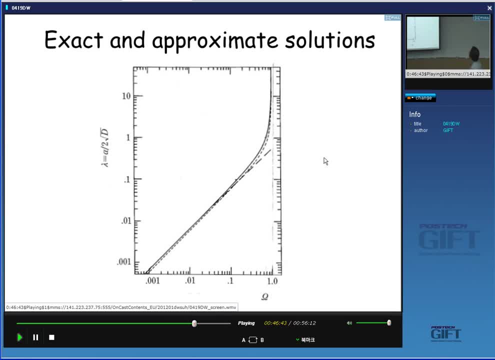 So you can see that the simplified approach is not that bad. Actually, it gives you quite reasonable way to evaluating the growth rate. Of course this is for the linear planar growth, But when we move to cylindrical Or spherical shape of the product phase, then the linear gradient approximation may not. 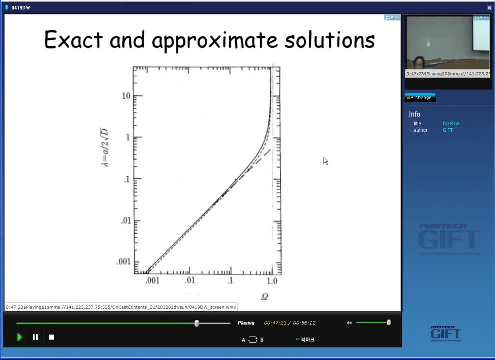 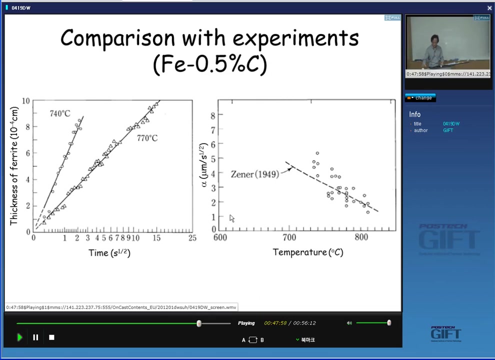 be a good choice. So you have to remember that the applicability of those kind of simplified approximation strongly depend on the shape of the product phase. So let's try with the ratio. The ratio is the inauguration phase. so how much is the? So? this is the experimentally observed, the power-relate constant. 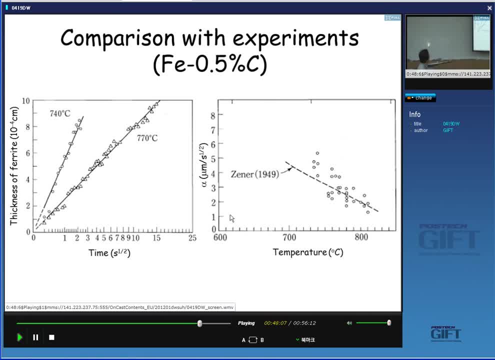 And this slope, as you can see, this slope is the rise. So the slope is the rise. The horizontal slope is low, The vertical slope is low. So the Newton's formula for getting the very high range, the horizontal slope is low. 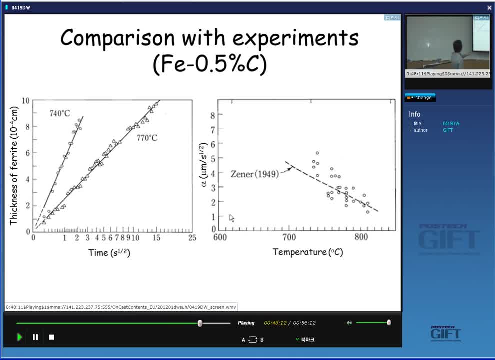 So if you can write a new formula and then apply to the dashight, you get six numbers. This x-axis is the scalar time and y-axis is the thickness which we put them to the side And you can see that between these two variables the linear relationship is observed, which 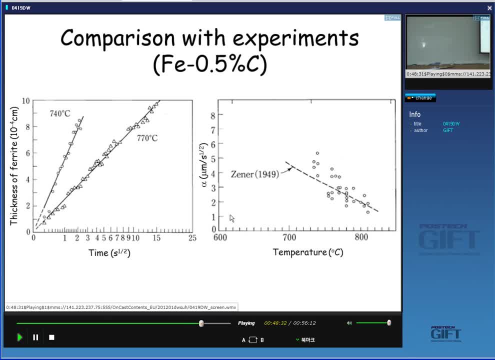 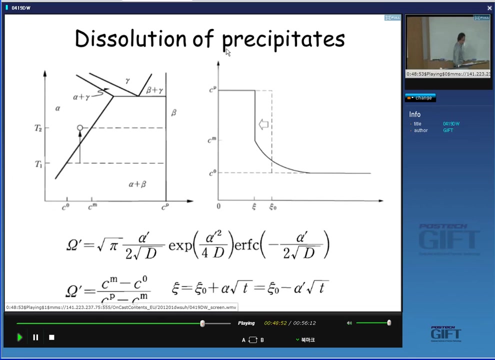 means that the alpha value can be regarded as a constant for given temperature, Which we expect from the calculation. Finally, I would like to say in a brief way, the dissolution. So far we have considered about the growth. But exactly, Exactly the same way you can treat the dissolution of the particle. 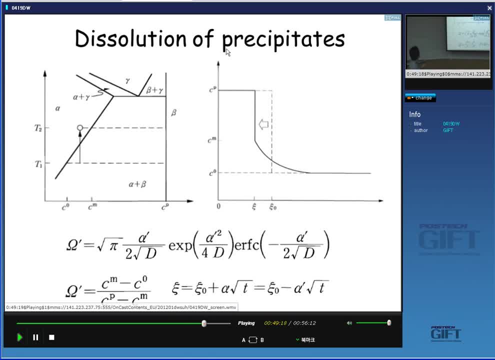 Here. at first let's see at temperature T. the system consists of alpha and beta, And then we hit the specimen into T2.. Then the particle starts to be solid Dissolved. The particle beta will be dissolved into alpha right. 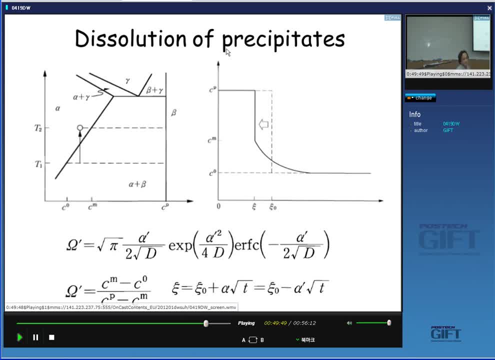 So dissolution rate, which, corresponding to the growth rate in reverse way, can be evaluated the same way. The first thing you have to consider is how the concentration profile will be. Here the dotted line represents the initial condition, Here the concentration of beta. 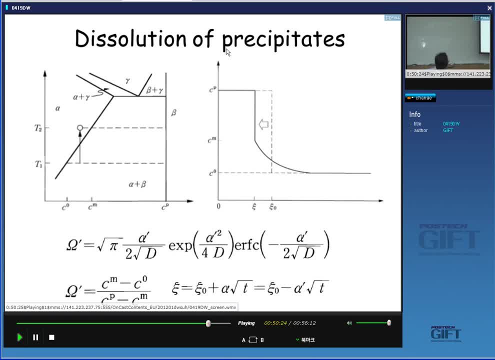 And here the concentration of alpha, which is given by the phase boundary at T, Then, when we heat up the specimen to T2.. Okay, Then the concentration profile will be changed. Okay, In a moment. The concentration profile will be changed like this one: 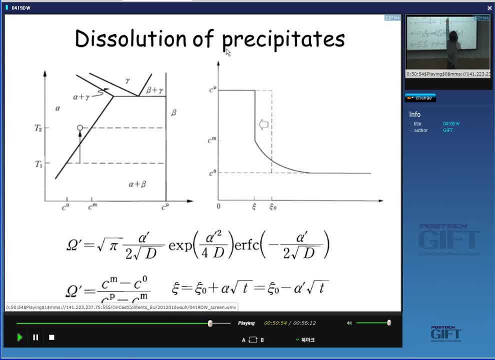 Whereas the beta phase dissolved. This kind of concentration profile will be developed. Okay, Okay, Okay, Okay, Here Here. CM is the concentration of alpha phase, which is equilibrium with beta at temperature T. Are you clear with it, The meaning of CM? 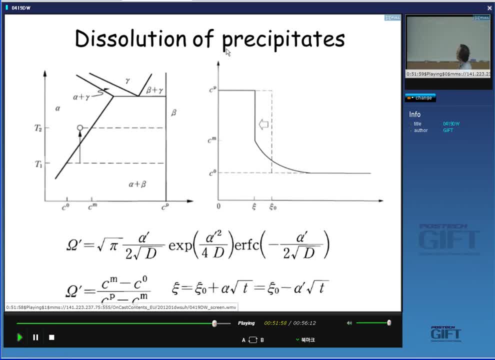 The position of CM in equilibrium phase diagram is here And this is the concentration, Okay, Of alpha, which is equilibrium with beta at temperature T2.. Okay, So you can expect this kind of concentration profile, and the exact solution of dissolution rate is given by this equation, similar to the previous one, when you evaluating this. 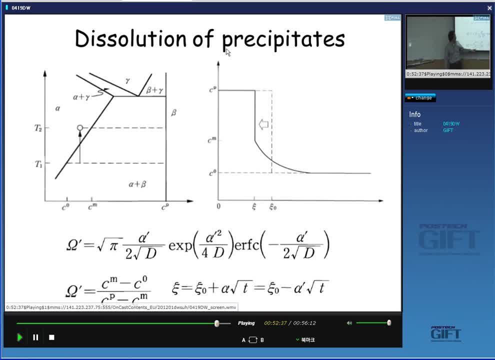 omega, which is given by this equation. Okay, So if you have this value- actually, this is constant when the temperature is fixed- then you can solve this equation to evaluate the position Here. the initial position, psi zero, And it will be decreased when time elapses, right? 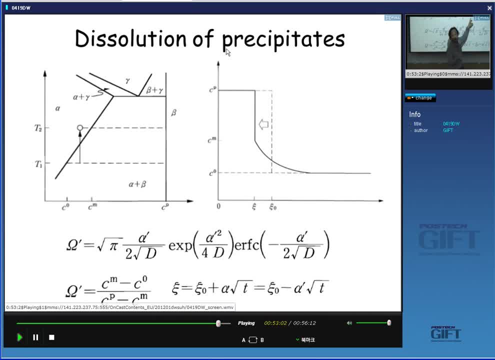 Because now we handle the dissolution. So the position of psi When time elapses Right, When you obtain alpha prime, you can evaluate with this relationship Okay. And also there is a way to treat this is as a linear, approximate approach. 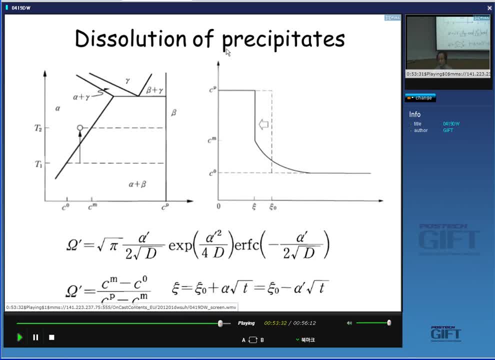 I will put this here, Okay. Okay, I will put that problem in the second problem set which I give you after the break. Okay, Any question? Is there any student who have class about 5 pm? Yes, Yes. 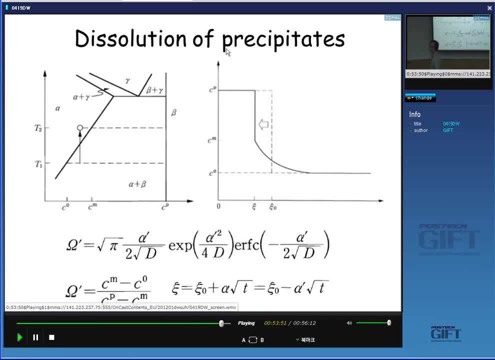 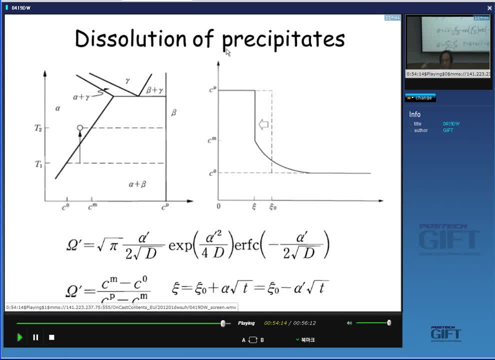 Yes, Yes, I do not know. No Wednesday, Like what I have learned all the time. What Thursday? I depends on day. How about Tuesday or Thursday? Korean Class. How about Monday? TM Lab, TM Lab. 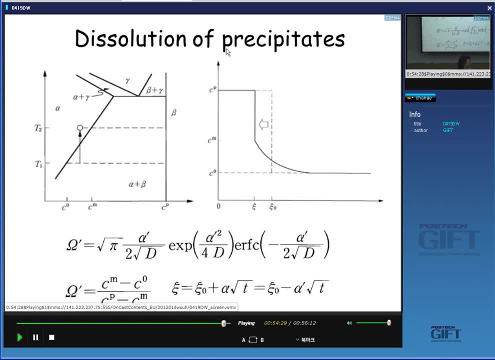 Okay, Tuesday, Wednesday, TM Lab Friday. Friday, Friday 5 pm. O But everyone, If everyone, happy I- bridge. Yes, I'm happy with it. Okay, Friday 5 pm. 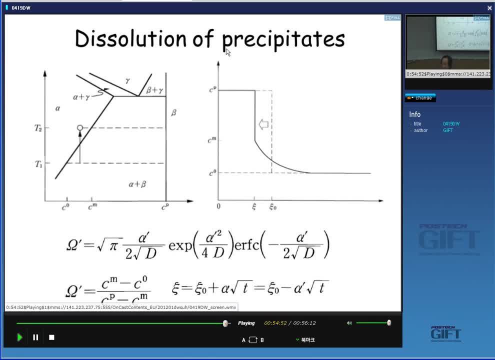 Earlier in the morning. I'm okay, but it depends on you. It's difficult to find time. How about when will be the TM lab? Monday and Wednesday, from 5 to 6.. Monday to Monday, Tuesday, Wednesday or Monday Wednesday. 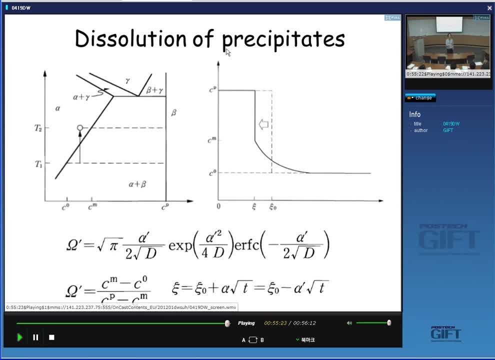 Monday and Wednesday. Then how about Tuesday? Tuesday 5 to 6.. Okay, then we can start at 6. Pardon: 6.15.. Okay, then how about the evening 7?? After the dinner: Tuesday: 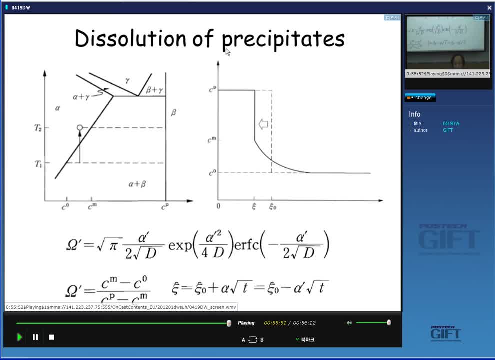 Just one makeup class, so you do not worry about it, And I will pick up The date and let you know, okay, And after I see the progress of the class, if I need to have a makeup class, then I will let you know the exact date, okay. Okay.